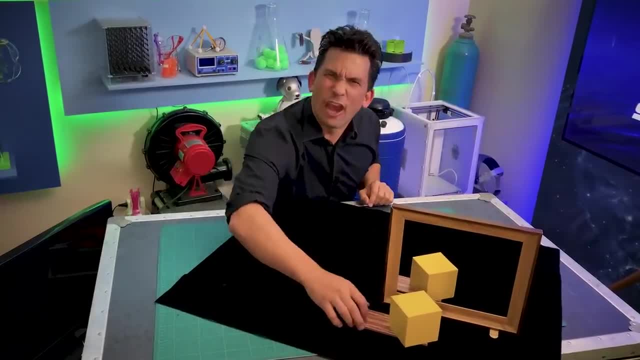 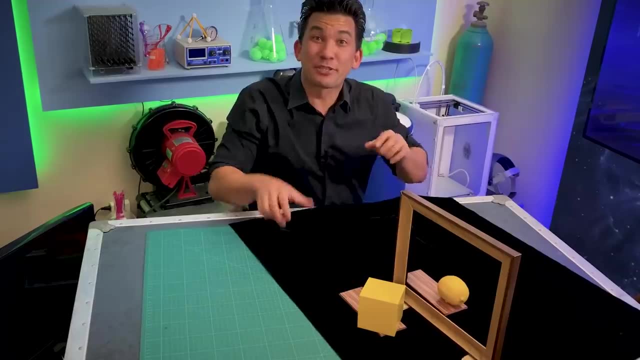 Today's episode is about reflections, Not necessarily how they work, but what can we do with science to make it look like a reflection doesn't work? That's right. today's episode is about a broken mirror, and how do we make an object's reflection different? 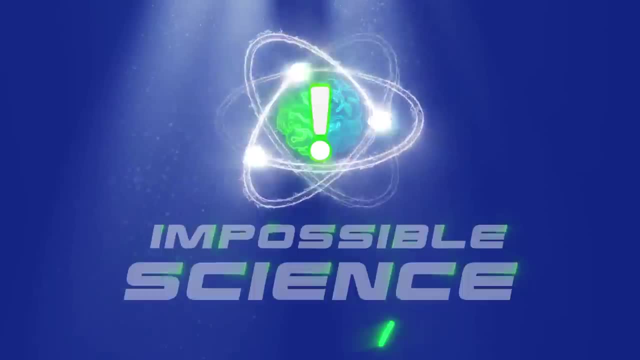 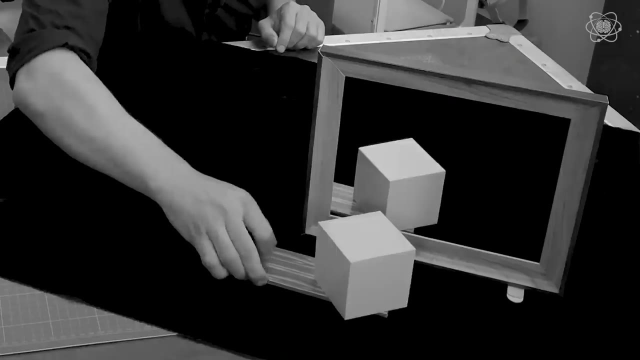 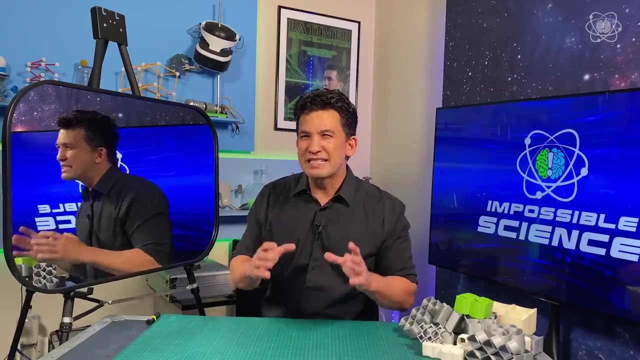 Welcome to Impossible Science. Hey everyone, it's Jason Latimer, world champion of magic, coming to you with another impossible science. Even though we're familiar with the subject of a broken mirror, where the reality is not matching, its reflection Turns out, even though it sounds impossible, a mathematical. 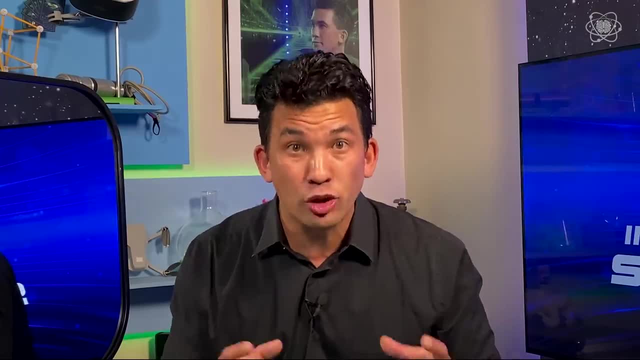 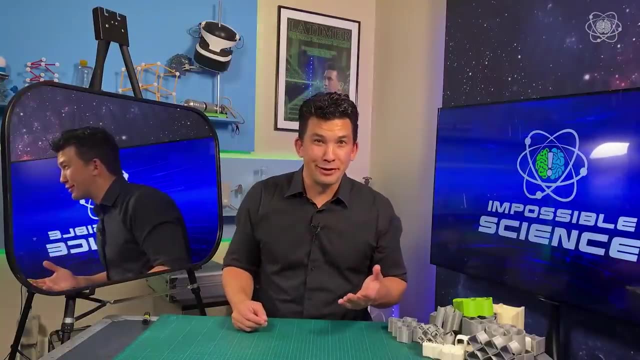 engineer, Professor Kokichi Sugihara, has figured out how to actually do this without it being a trick, And it uses what's called an ambiguous figure. What is an ambiguous figure? Well, an ambiguous figure is an object that has two images in the same image. It means it can. 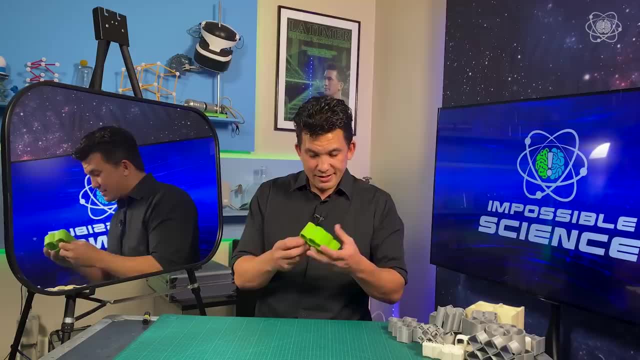 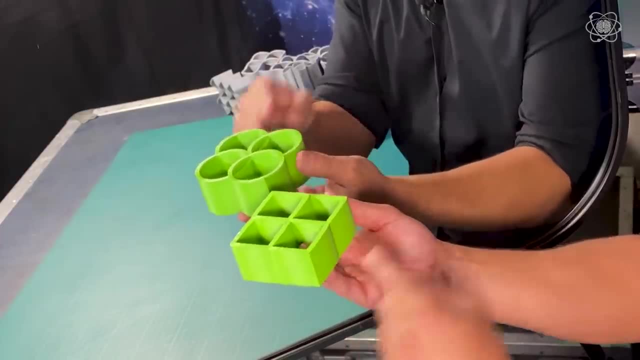 actually be two different shapes from two different vantage points. This is an ambiguous figure. If I put this up to the mirror right now, you can see the squares in the foreground. but look in the mirror. Isn't that crazy? There's squares in reality. 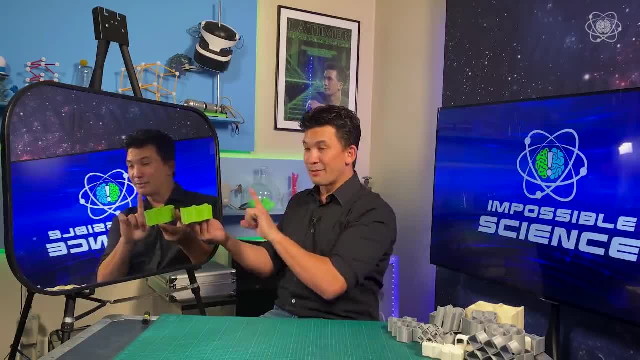 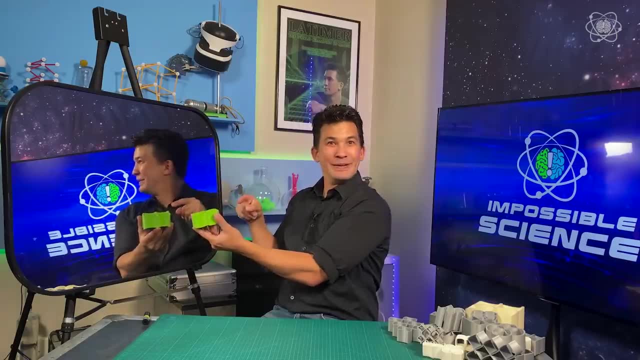 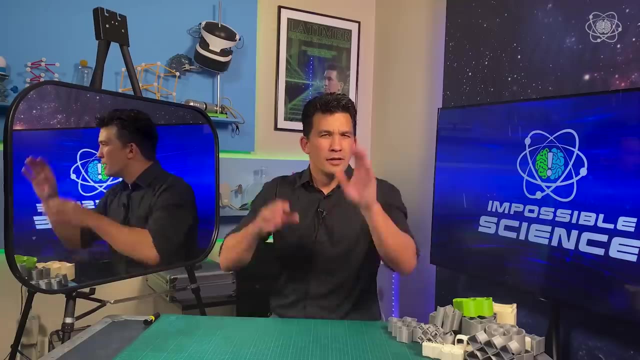 there are circles in the mirror. This is where it gets nuts. I'm going to flip this around, no sleight of hand. Now you've got circles in reality and you've got squares in the mirror. What Circles, Squares, Squares, Circles- Now, if you're anything like me- and reflection. 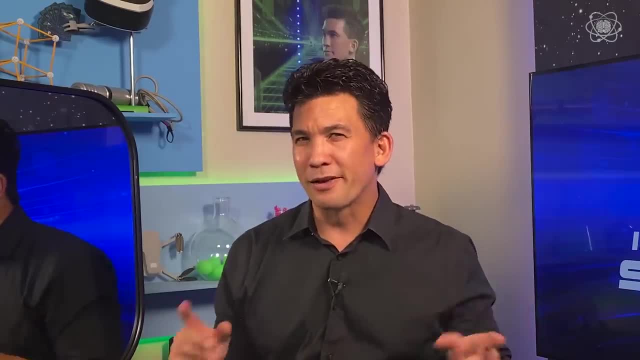 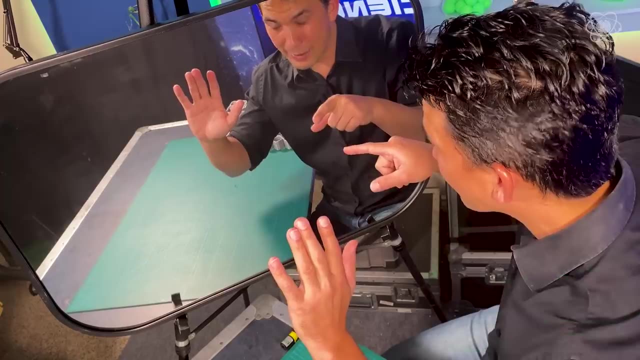 is kind of confusing. just go, why do mirrors reflect left and right but not up and down? See, you can look in the mirror and go. I can wave my left hand and my reflection's right hand waves back. I can wave my right hand and my reflection's left hand reflects back. And if I tilt my head? 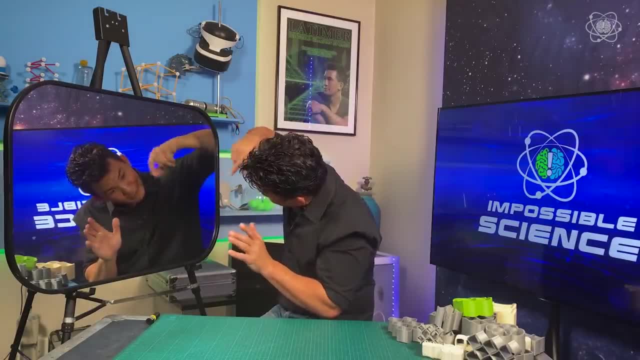 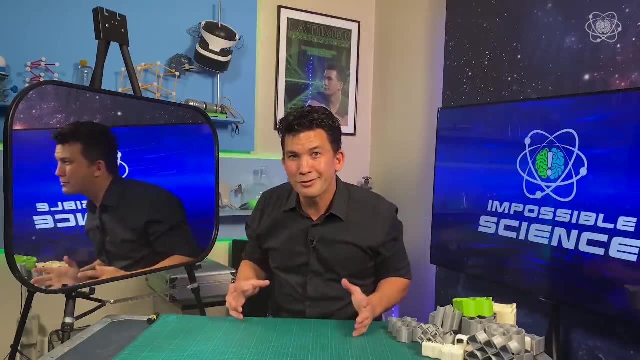 the same thing happens. My right hand is left hand in the mirror and my left hand is my right hand in the mirror, So it's switching left and right And yet when I tilt back up it's not switching up and down. How does the mirror know? Mirrors reflect front to back. 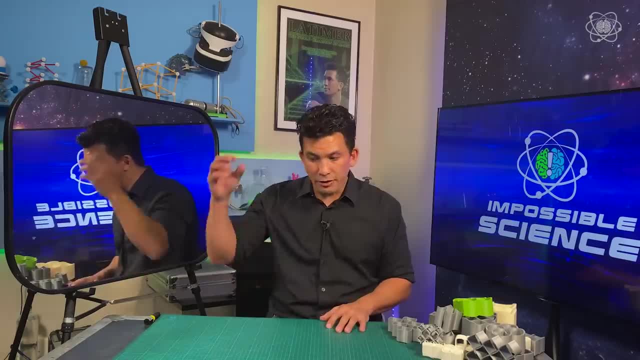 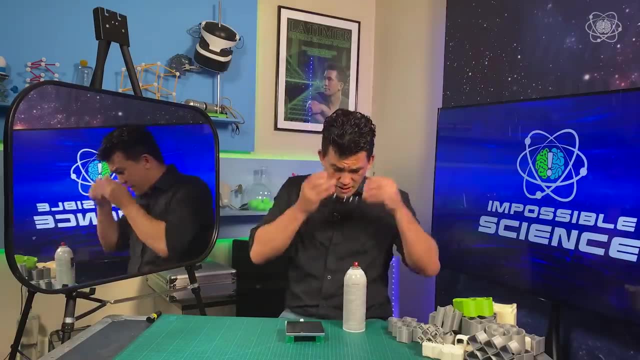 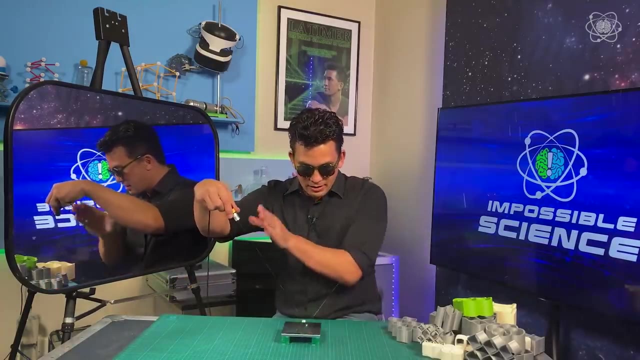 To really understand this, you have to understand the law of reflection. The angle of light coming in is equal to the angle of light coming out. I'll show you with an experiment With some safety glasses and some smoke, so you can see it. If you look at this, the laser coming in. 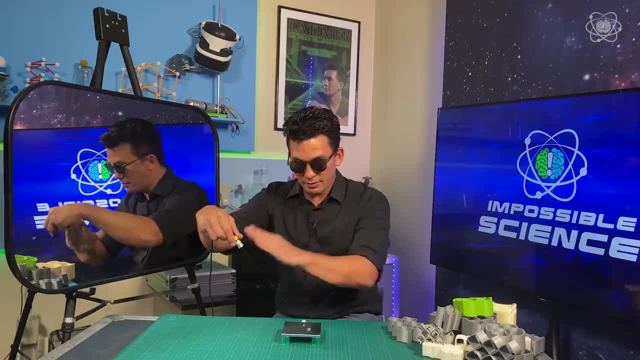 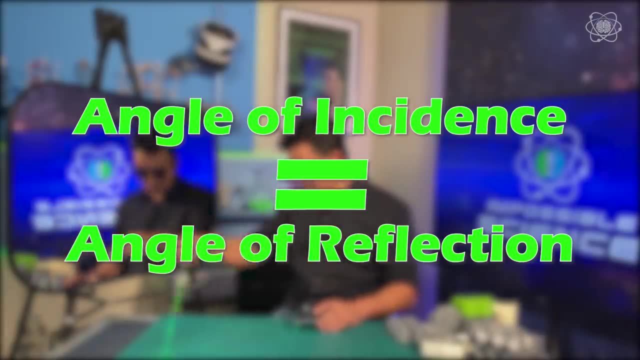 bounces off. If you imagine a perpendicular line right here, the angle to this laser is the same angle as it's reflecting out. The angle of incidence is equal to the angle of reflection. Now why is that important? Because with a mirror, all the light coming in is simply retracing its. 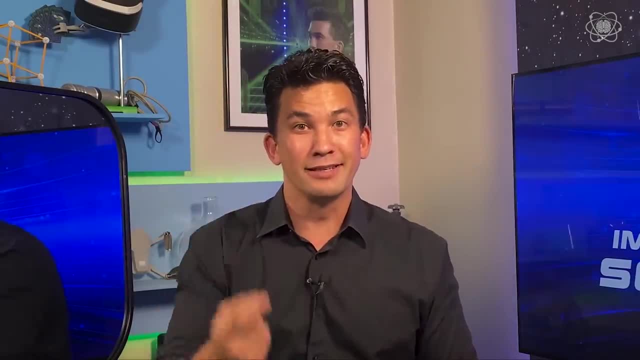 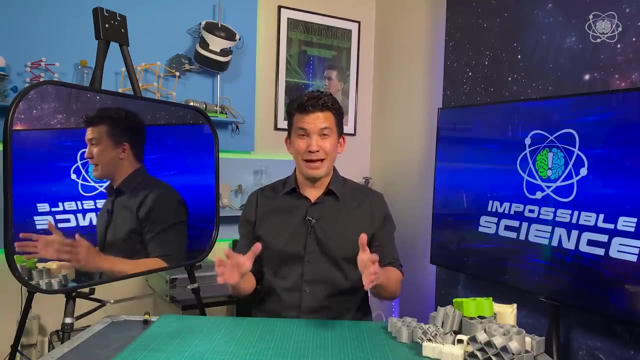 steps on the way back out. Going in at 90 comes back out at 90. Angle of incidence equals angle of reflection. So if you're wondering, if a mirror doesn't reflect left or right- and it really doesn't have any magic powers- why does a vampire not show up like in Hotel Transylvania? Well, 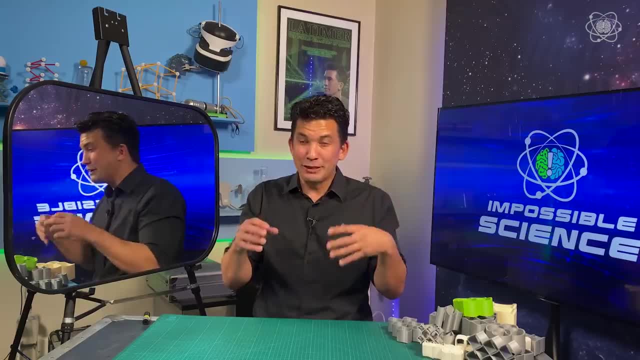 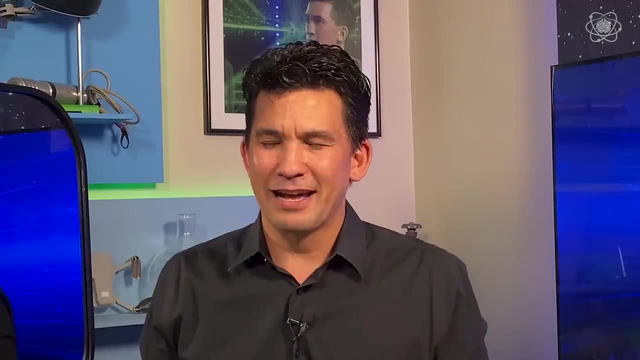 mainly because a lot of people think that vampires must be transparent And so the light travels through it, So they won't have anything to reflect off a mirror, And that's exactly what I'm going to show you here. But that's not necessarily true, Because if they were transparent, you wouldn't see. 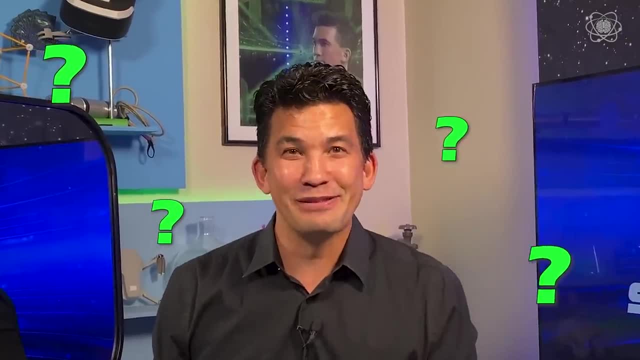 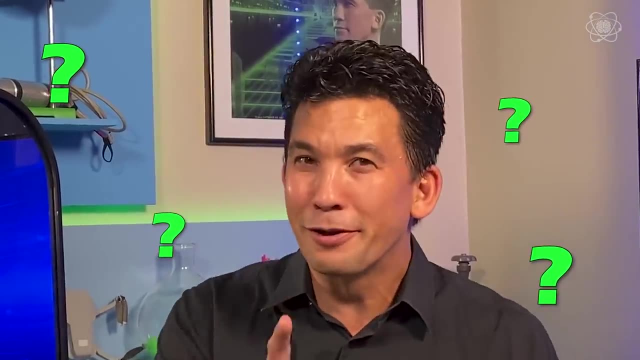 them even if there wasn't a mirror. I have a question for everybody: Why are the vampire's clothing vanishing too in a mirror? Like I get it if the vampire is magical, but their clothing should show up in the mirror. Or how did he do his hair in the morning? How do you shave? 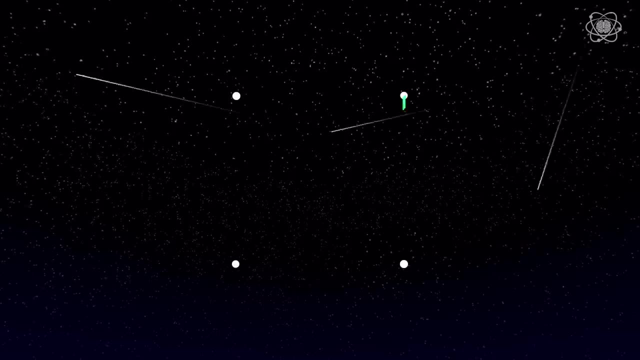 Okay, back to the science. If you were to go outside and look at the stars, you might find four bright stars that you could use to trace out a square. While this may make a difference to us, it's very likely that the actual position of those stars do not form a square from. 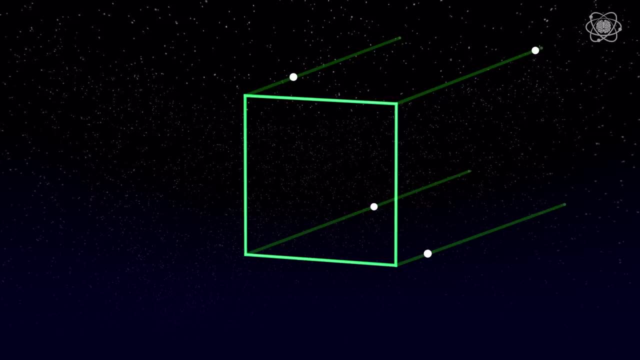 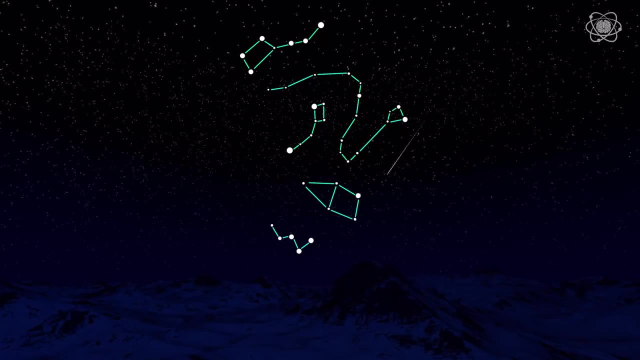 any other perspective, Each of those stars could be closer or farther away, In fact, all of our constellations that we hold dear to our heart and our imagination. they are not on a flat plane, Even though they look like it. our constellations only appear as those shapes. 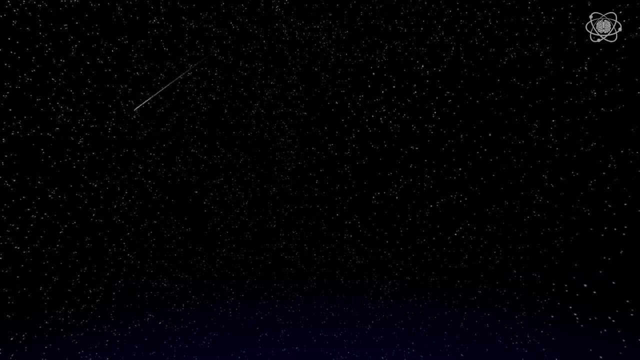 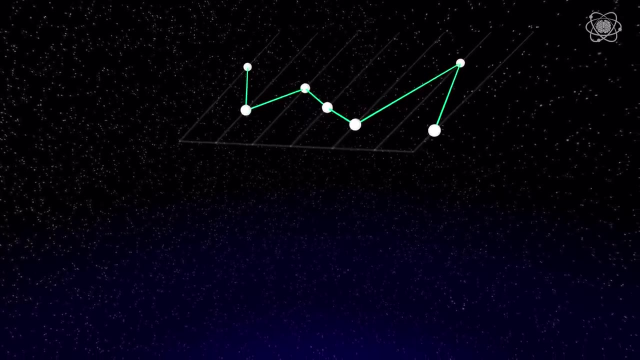 from our very distant vantage point, If we imagine a line made up of individual points, it's easy to visualize how each of those points could be closer or farther away. So from one perspective, it's possible to have an infinite amount of ways to. 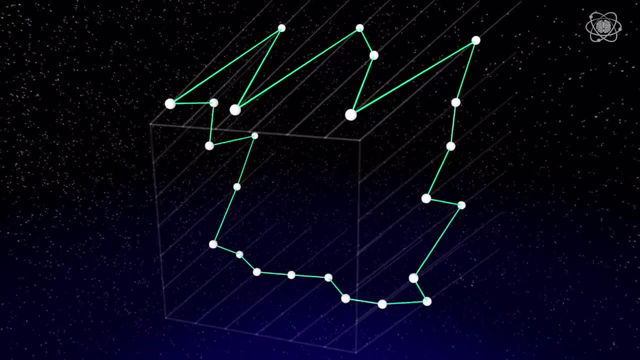 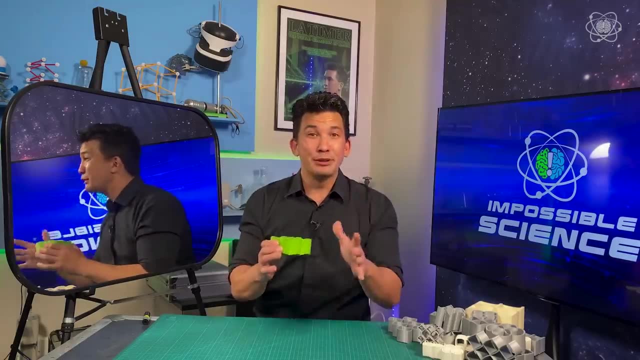 draw a line, And since a 2D drawing is a flat image made up of multiple lines, you could see how there could be an infinite amount of ways to draw that image. When I first saw this, it blew my mind. Luckily, I was able to get a hold of Kichi Sugihara and actually ask him what is going. 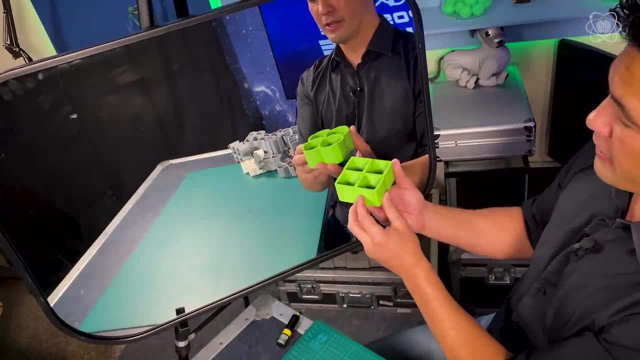 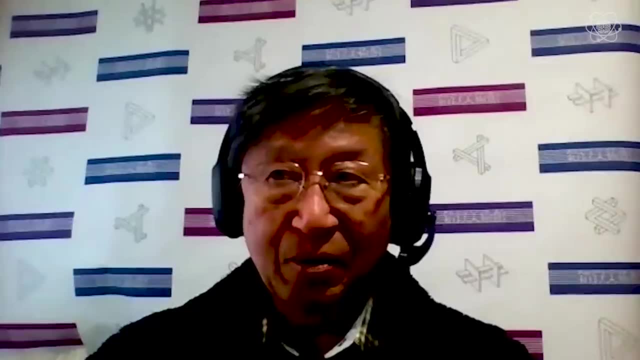 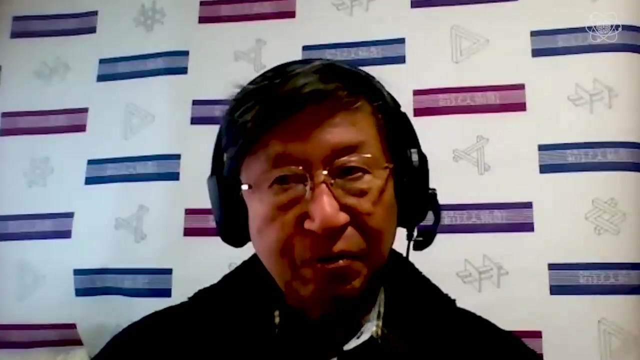 on. Why am I able to see something different than its reflection? Professor Kokichi Sugihara, welcome to the show. So where did the idea come from? Okay, first of all, I was doing research on computer vision, in which one of my topics is to 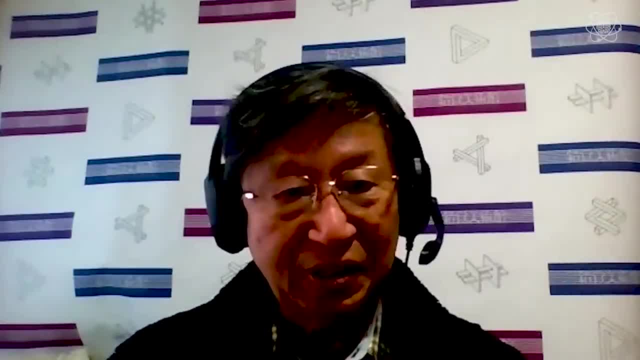 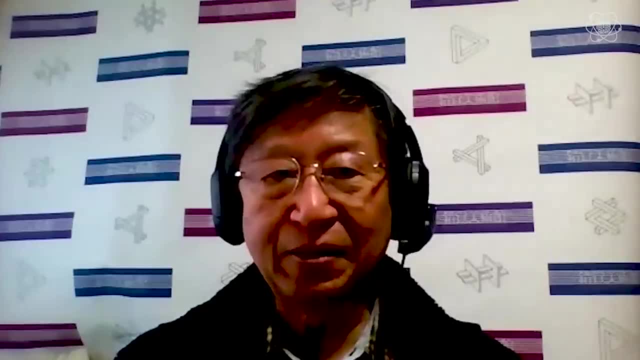 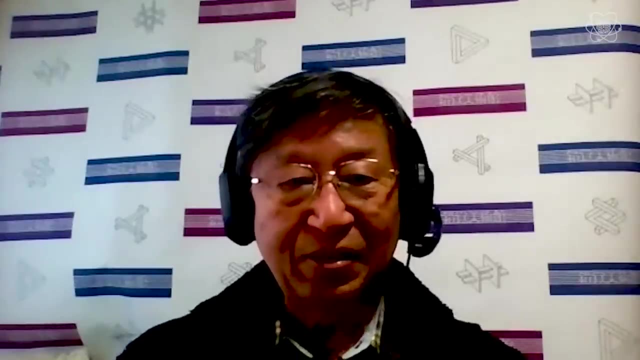 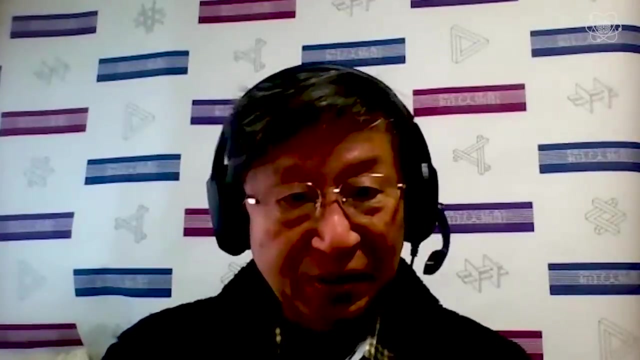 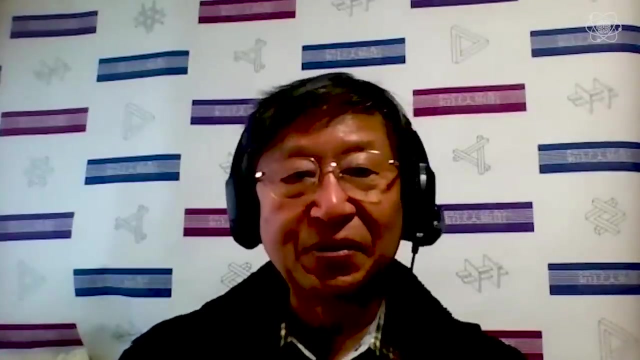 deconstruct three-dimensional objects from two-dimensional single images And mathematically the single image cannot represent a 3D object uniquely. There are many, meaning that the same picture corresponds to infinitely many possible 3D objects. When we have two desired shapes circular from the first viewpoint. 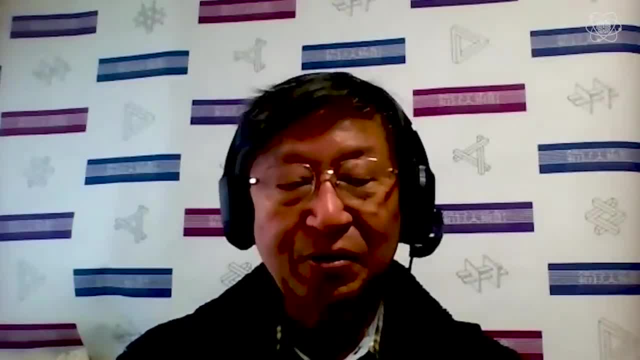 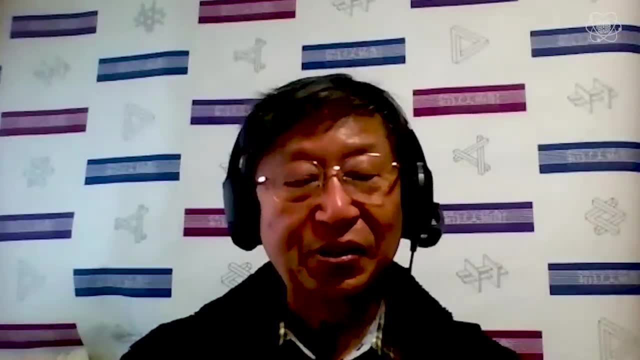 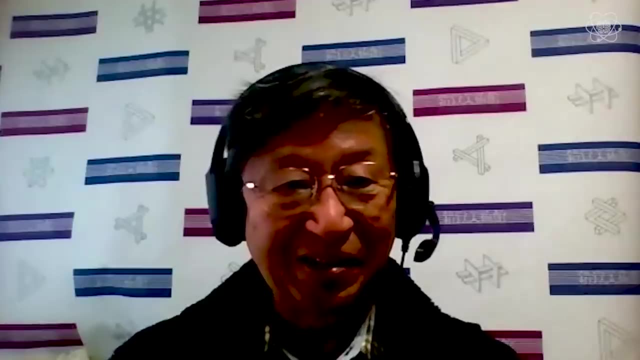 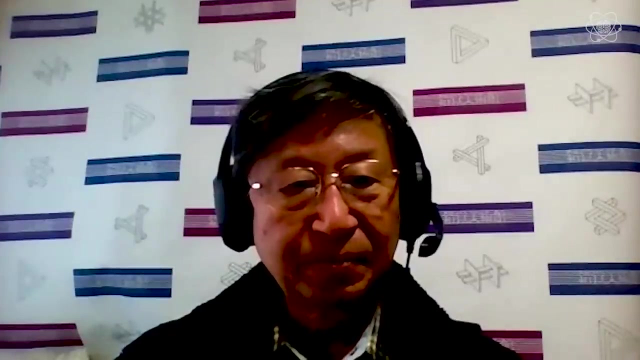 rectangular. from the second viewpoint, then we can construct two equations and combine them and solve it, And if it has solutions, that is the object we want to get. In that way I found the circular rectangle cylinders. Am I right in saying you have one equation looking straight out and then you have another equation? 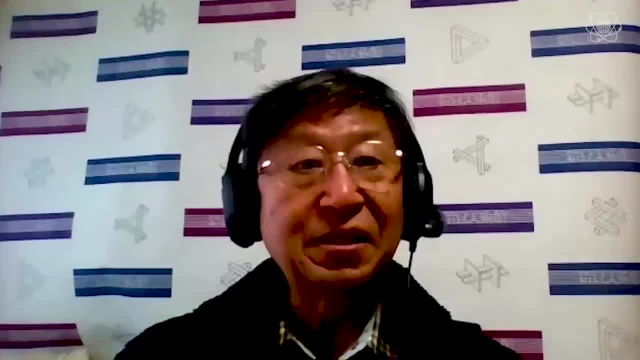 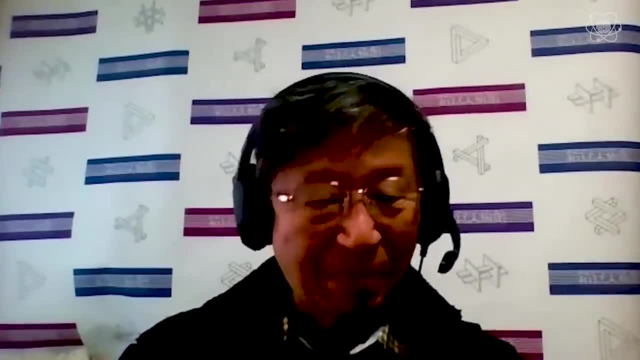 and there's a point that solves both equations. Yes, yes, yes, So it's a kind of triangulation. In order to find the point in space, we can specify the two appearances from the two viewpoints. That is a triangulation. And 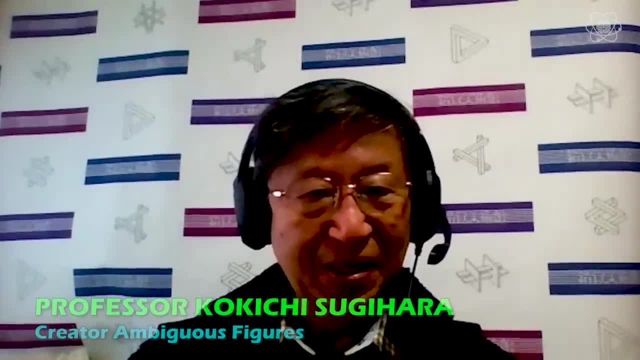 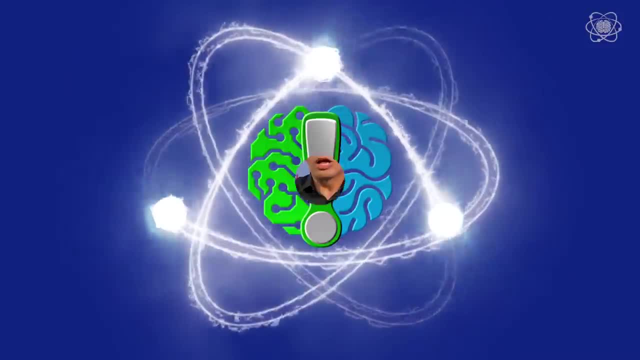 then you arrange it by setting it in the right place and then you can draw the two-dimensional shape. So it's a kind of triangulation. But if we are extending that principle to a set of points, we get that kind of object. Professor Kokichi, thank you so much. 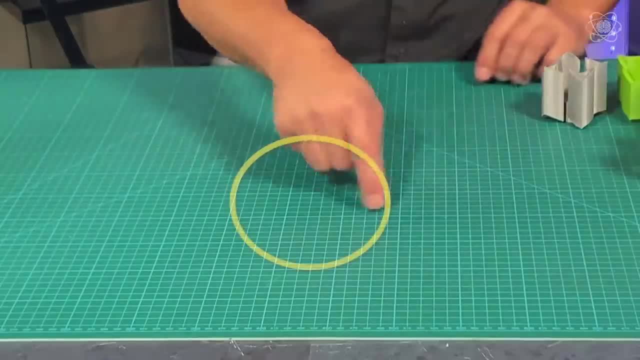 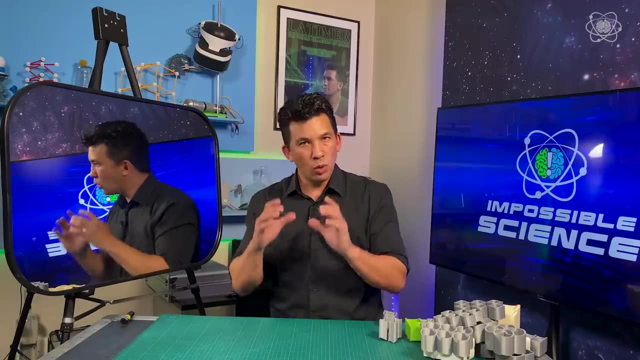 Thank you. Now, once you understand that you could draw a two-dimensional shape an infinite amount of different ways, well then, ambiguous figures start to make sense. See, imagine, a circle on the table, and from my point of view, there's equations that make up a circle. 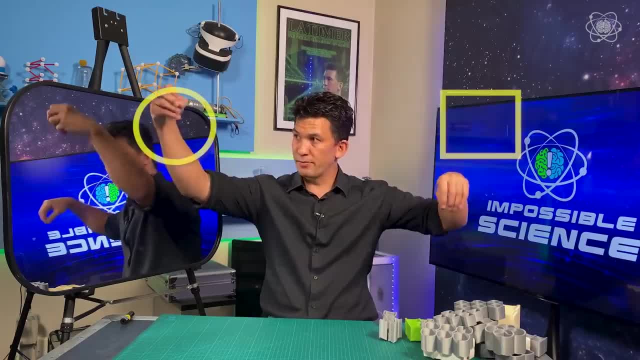 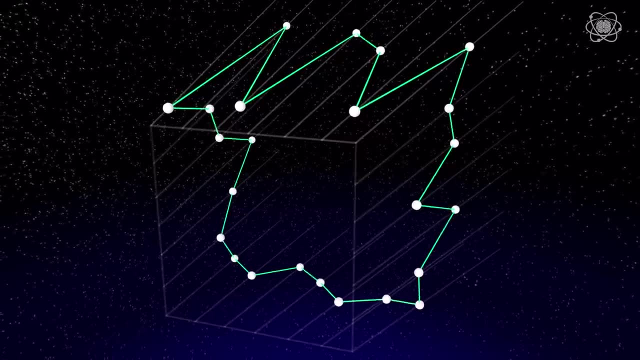 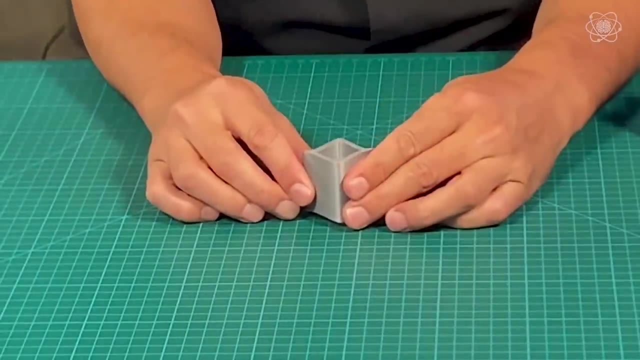 from my point of view, Now make those two equations from this side of a circle, interfering with these that make a square, and given the infinite amount of possibilities, there's points that are satisfying both equations at the exact same time, and those points make up the ambiguous figure, which is why you see.